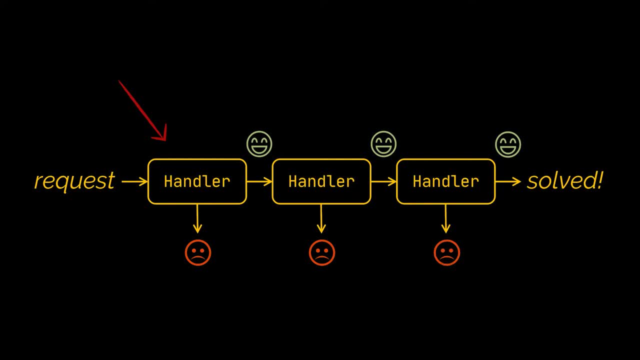 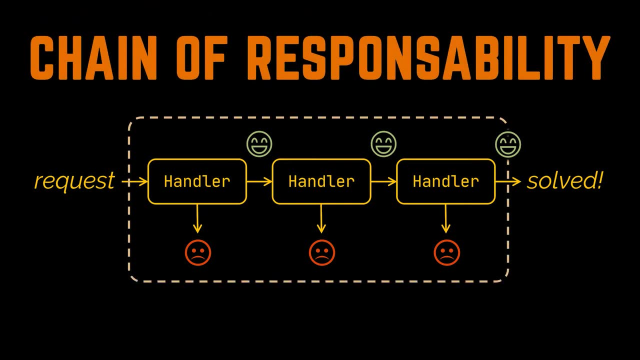 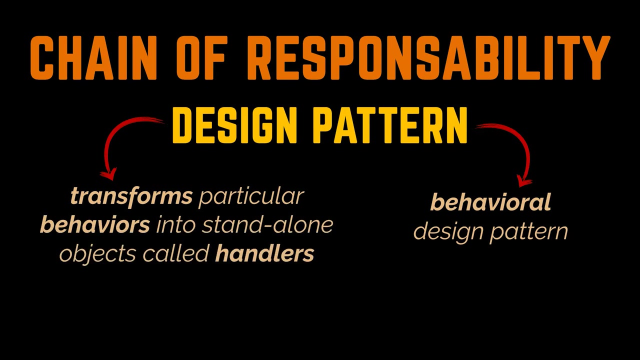 pass the request. A handler can pass the request further down the chain and effectively stop any further processing. This example and many others are perfect real-life analogies to the chain of responsibility design pattern. This pattern is a behavioral design pattern that lets you transform particular behaviors into stand-alone objects called handlers. Then, upon receiving, 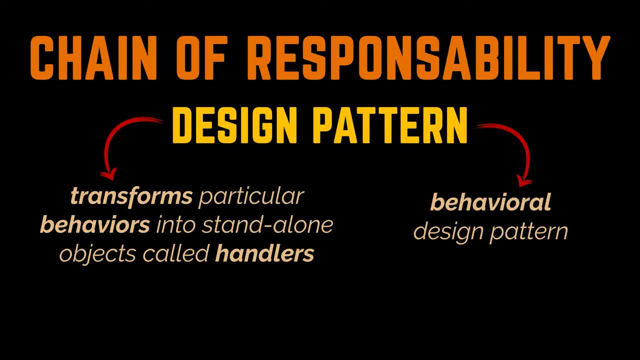 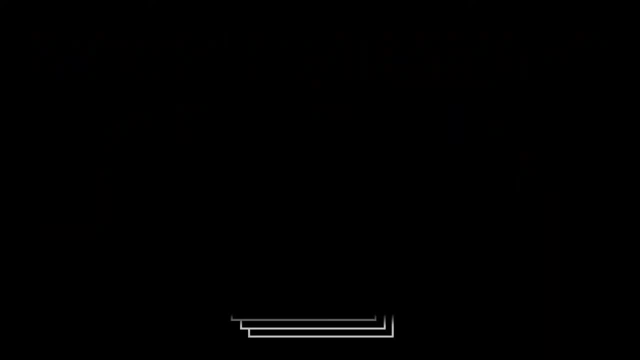 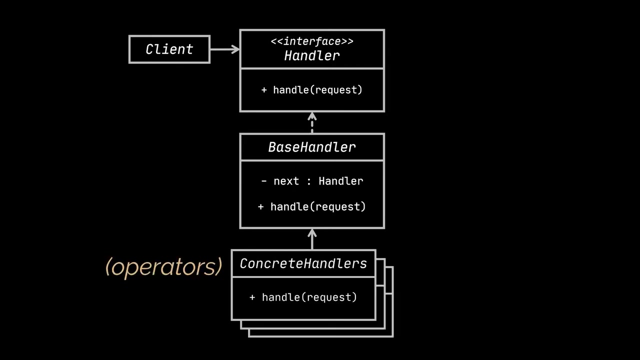 a request. this request will pass along the chain of handlers, where each one can decide either to process the request or pass it to the next handler in the chain. 🎵. Alright, before we try to implement this pattern by basically analyzing the planetary downstream倒 계. 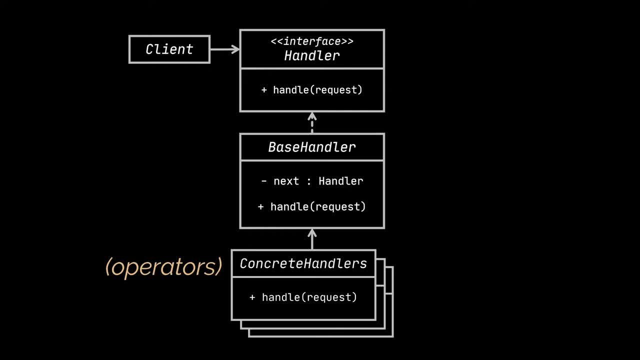 chain that then sticks to it. let's look at a more practical example 🎵. These classes contain the actual code for processing requests. They are usually self-contained and immutable, accepting all necessary data just once via the constructor. These concrete handlers implement the actions contained in tango and mind states, And this is the first. 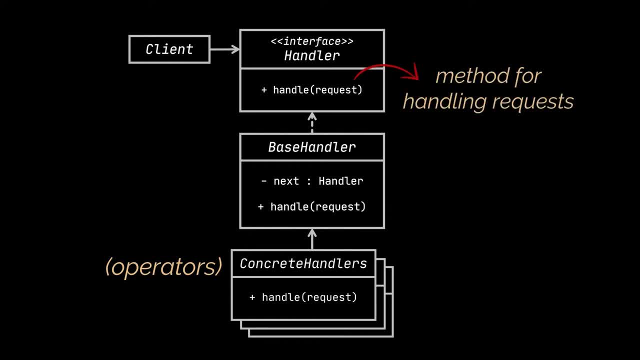 example, which」 implement a common interface, the handler interface. It usually contains just a single method for handling requests, but sometimes it may also have another method for assigning the next handler in the chain, just like a linked list. The base handler is an optional class where you can put the boilerplate code, that's 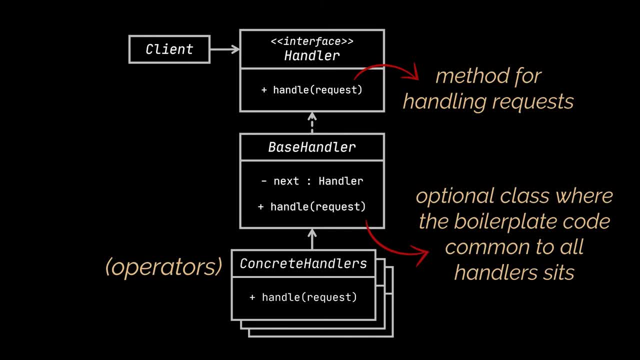 common to all handler classes. Usually, this class defines a field that stores a reference to the next handler. Finally, the client composes the chain of handlers. This can be done once or dynamically, depending on the application's logic. Additionally, the requests he composes can be sent to any handler in the chain. It actually 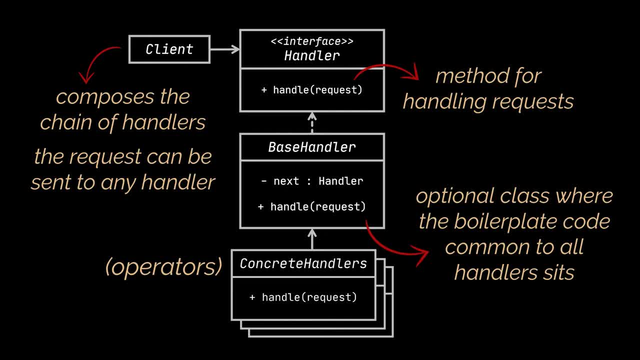 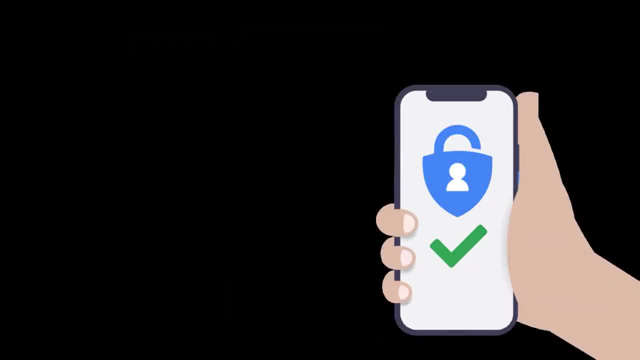 doesn't have to be the first one. Let's go ahead and try to implement the chain of responsibility pattern. To do this, suppose you are working on an authentication app and for a user to log in into our platform, he or she must pass several checks. 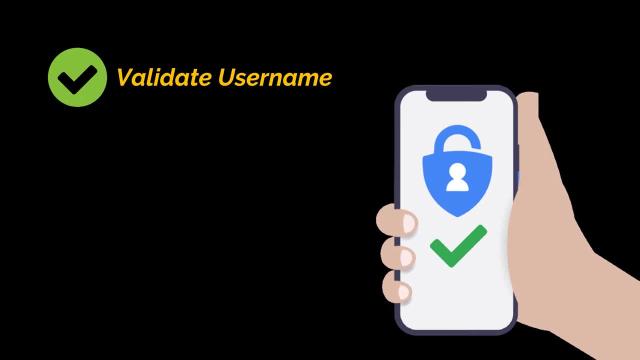 First, we need to make sure that the username entered indeed exists in our space. Next, if the username exists, we need to verify that the password entered by the user matches the corresponding password tied to this username And, if not, we must alert the user that the password entered is incorrect. 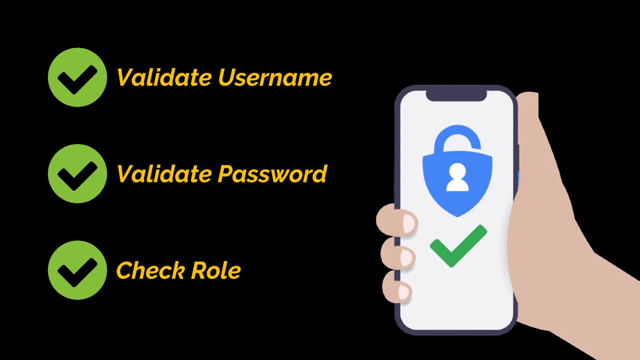 Finally, if both these checks are validated, we need to go over the admin users of our application, because if the user that is trying to log in is an administrator, we perhaps may have to enable additional admin pages for him or grant him security. 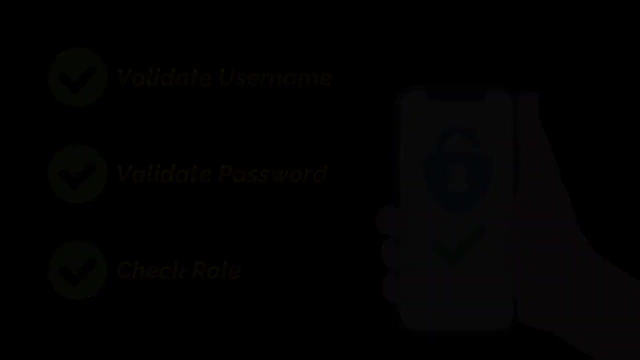 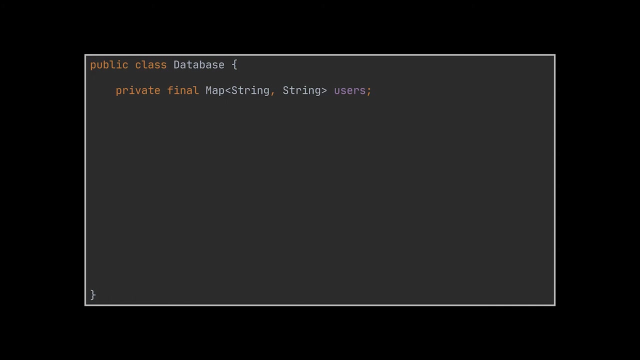 Let's start off the implementation with a database class. This one will simulate the database storing the usernames and passwords of our users. with the help of a HashMap, You could have established a connection with the real database, but I am not going to waste time doing it here, as it isn't the main target of our video. 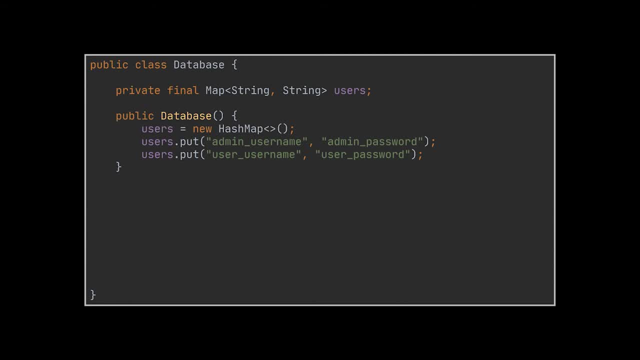 So in the constructor we are going to insert a couple entries inside the map and we'll add to this class two helper methods, one for each of the checks we need to do. The first one will check if the user has logged in. 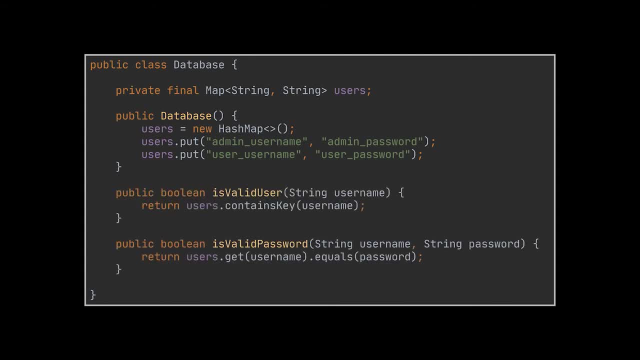 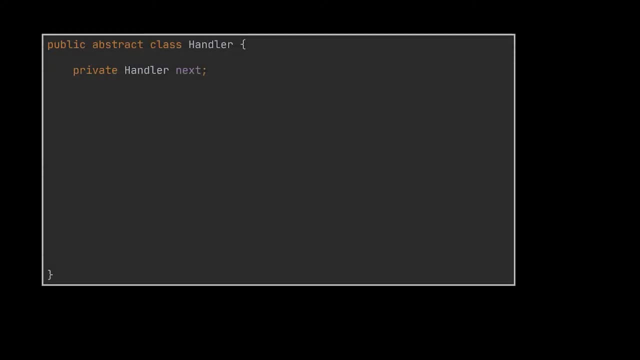 The second method will make sure that the password provided corresponds to the username the user has entered. Now let's go ahead and create the handler abstract class. This one, as we previously mentioned, will store a reference to the next handler in the chain. 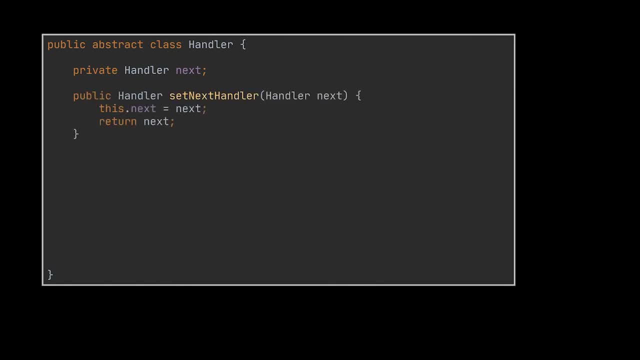 It will also define a method that allows us to assign this reference like a setter for the next handler. Moreover, this class will contain an abstract method, the handle method. This method will be implemented by the concrete handlers, where each one will define the condition. 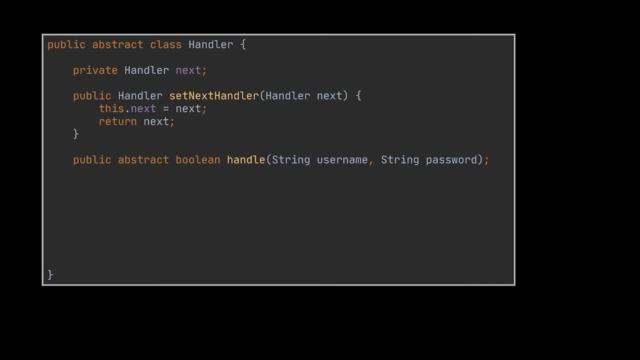 based on which the user is eligible to access our application. You could go ahead and move this method to an interface and make the handler class implement this interface. However, in this case, and as we saw on the structure diagram of the chain of responsibility, 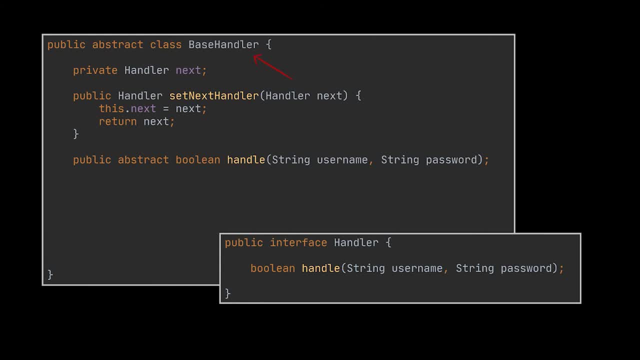 the current handler class will become the base handler and the interface should be named handler. as we previously discussed, We are going to proceed without an interface and add to the handler abstract class one last method. This method will house the convenience of the handler class. 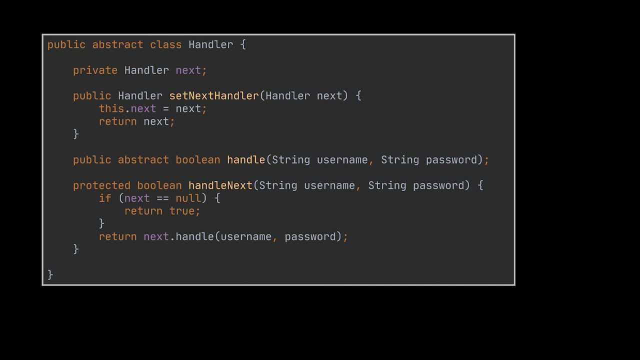 The handler class will be the default behavior of a handler, which is to forward the request to the next object unless there is none left. Concrete handlers will be able to use this behavior by calling the parent method. Speaking of concrete handlers, we have three. 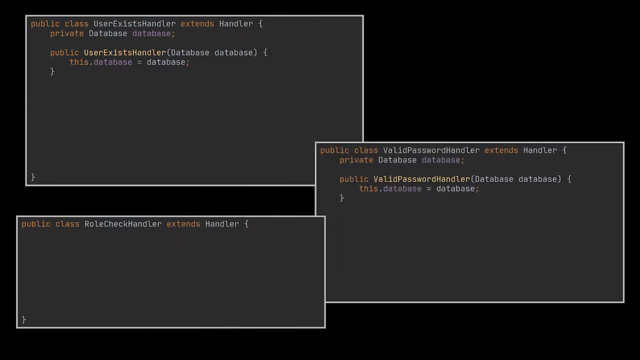 The user exists handler, the valid password handler and the role check handler. Each one of these handlers must implement or override the handle abstract method. Inside this method, we will have a condition that calls the corresponding helper method defined at the level of the database class passed to the constructor.